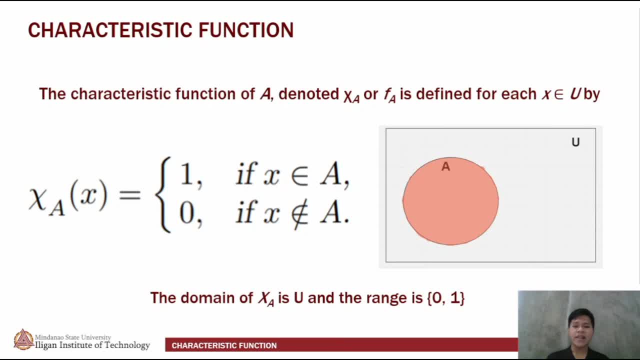 The characteristic function of A denoted with a capital letter x and a subscript a, or a small letter f and a subscript a is defined for each x that is an element of U or the universal set by having this Red. 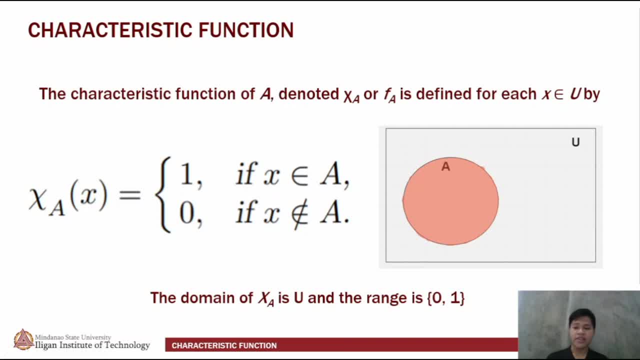 Red as the characteristic function of an element x in a given set A, which has two possible outputs: one if x is an element of A and zero if it's not. The domain of the characteristic function of a given set in this case is A, is the universal set U, and it will always be the same case with the other given set. 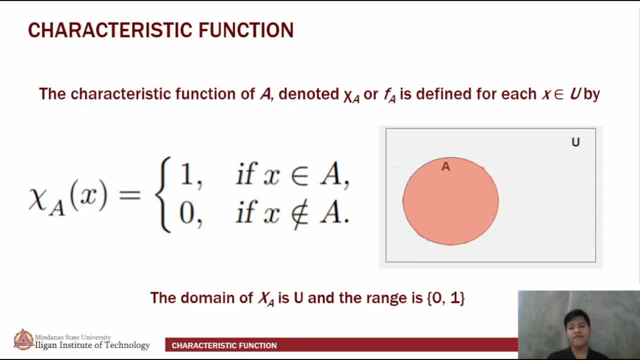 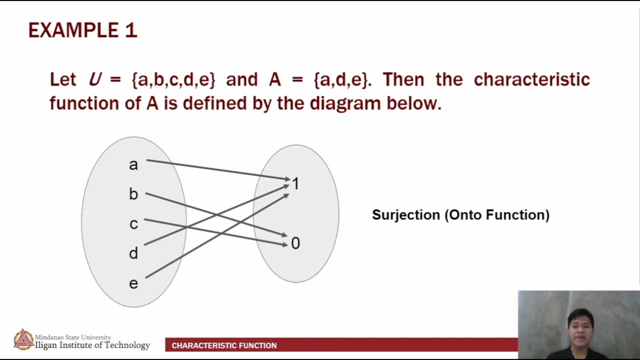 The range is from 0 to 1.. And for the characteristic function, we will be only using the integers 0 and 1 for the range. Here we have our first sample problem. Let U be a set containing the elements A, B, C, D and E and A as a set containing the elements A, B and E. 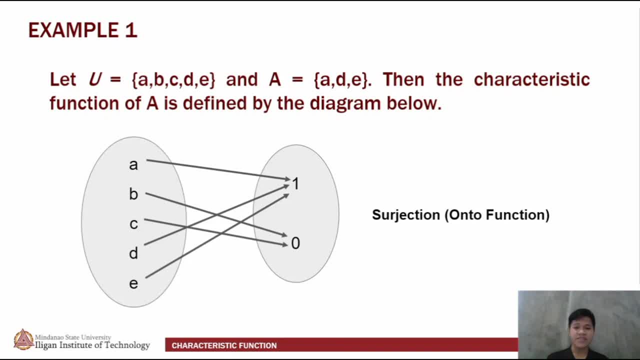 Then the characteristic function of A is defined by the diagram below. We can see that the letter is A, A, B and E are matched with the value 1, whereas B and C are matched with the value 0. It is because the elements B and C are not elements of the set A, which compose only of the elements A, B and E. 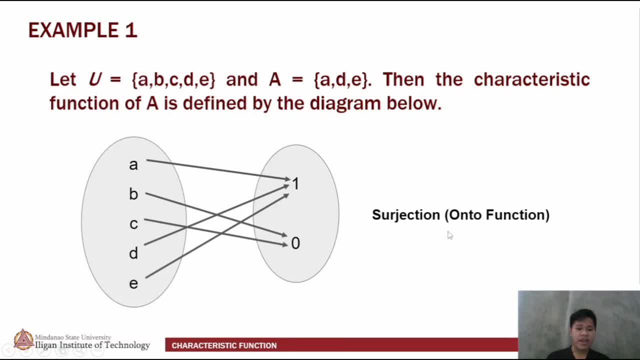 And on the right side it says Sejection. If we recall our previous lesson from the previous reporter, a Sejection or an Onto function is a function wherein every element on the right side- our range in this case- has at least one element matched on the left side, or the domain. 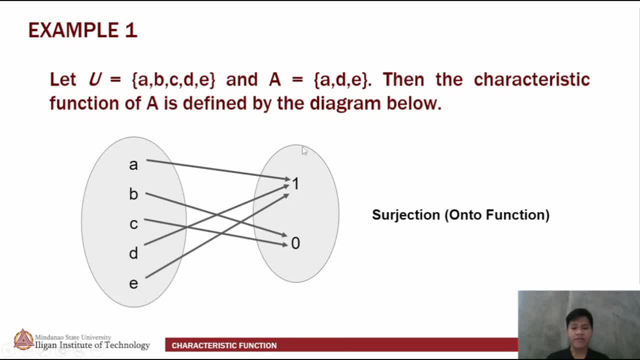 We can see on the diagram that every element on the right side or this range- the 0 and 1, are connected to at least one element on the left side or on the domain. As you can see, 1 is connected to A, B and E and 0 is connected to B and C. 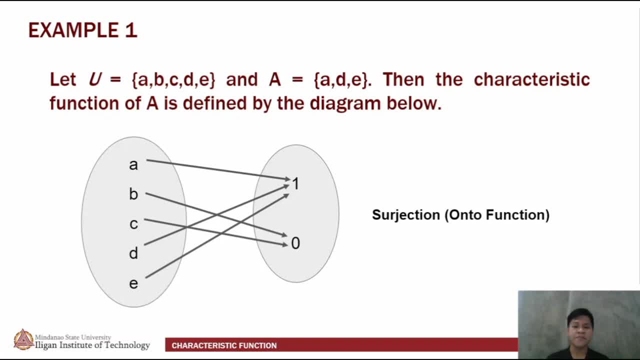 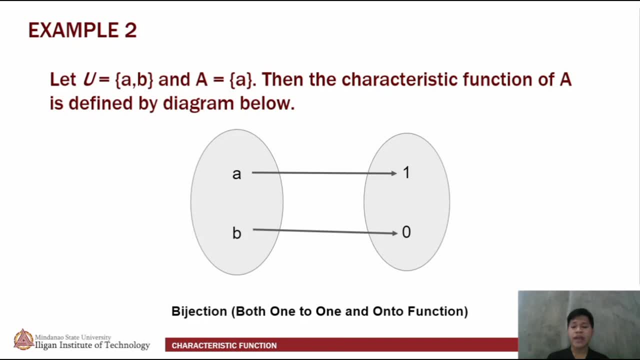 That's why we identify it as Sejection or an Onto function. So for our second example, let U be a set containing the elements A and B and set A containing the element A only Then the characteristic function of A is defined by the diagram below. 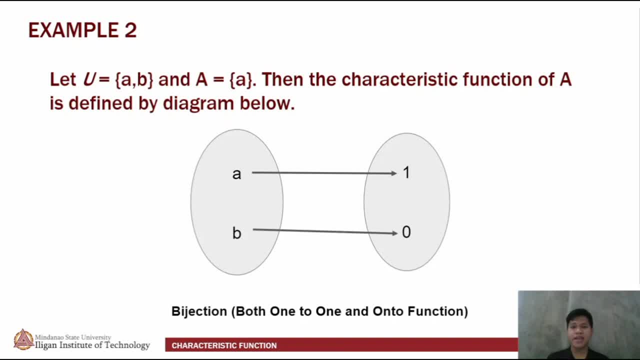 We can see that A is matched with the value 1, and B is matched with the value 0. Since only the element A, this one, is under the set A. This diagram is a Sejection, since it is clearly seen on the diagram that it is a 1-to-1 function and at the same time an Onto function. 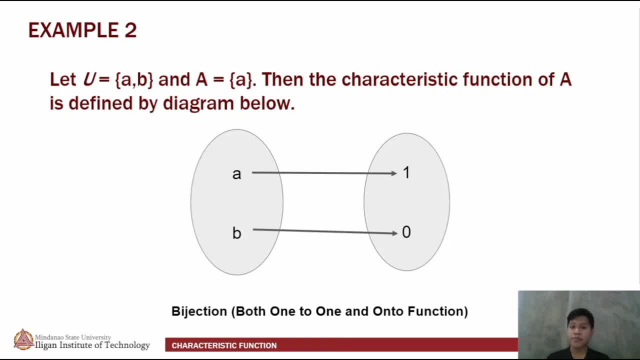 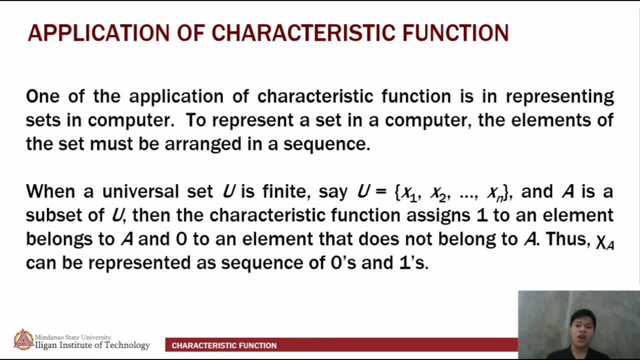 Just like how we remember it from our previous discussions with the previous reporters. Now for the application. One of the applications of the characteristic function is in representing sets in a computer. To represent a set in a computer, the elements of the set must be arranged in a sequence. 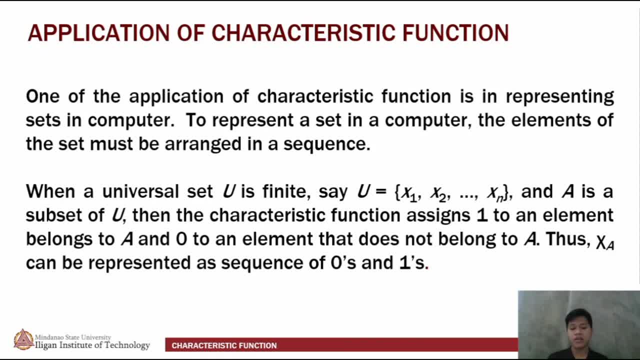 Aside from using 0s and 1s to represent ordinary numbers in binary form, it is also used to identify true or false in computer logic, wherein we use 0 for false and 1 for true When a universal set, U, is finite. say, U is a set containing 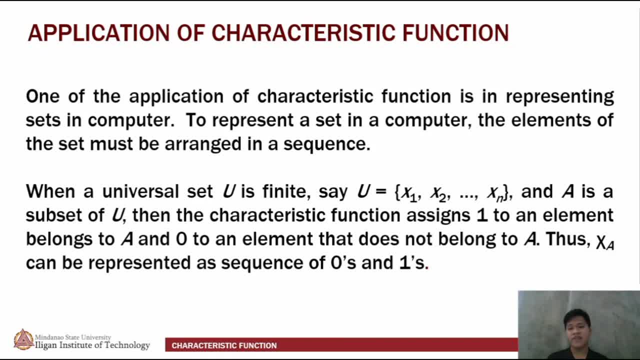 the characteristic functions of values 1,, 2, and so on and so forth. and A is a subset of U, then the characteristic function assigns 1 to an element that belongs to A and 0 to an element that does not belong to A. 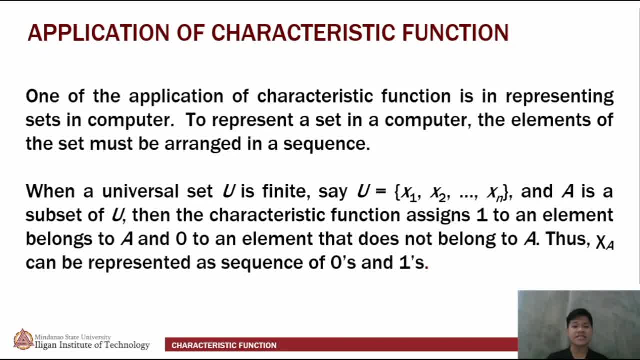 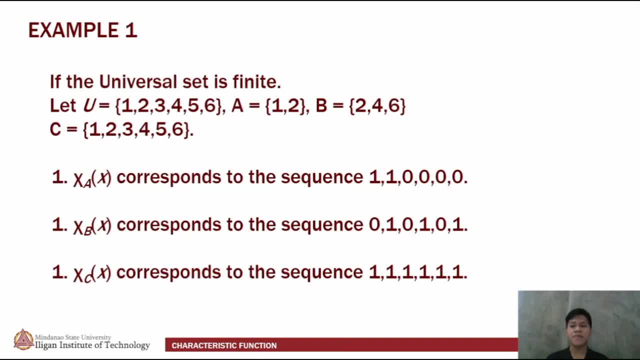 Thus the characteristic function of A can be represented as a sequence of 0s and 1s, And we will find out about it on the next example. If the universal set is finite, then we let U as a set containing the elements 1,, 2,, 3,, 4,, 5, and 6,. 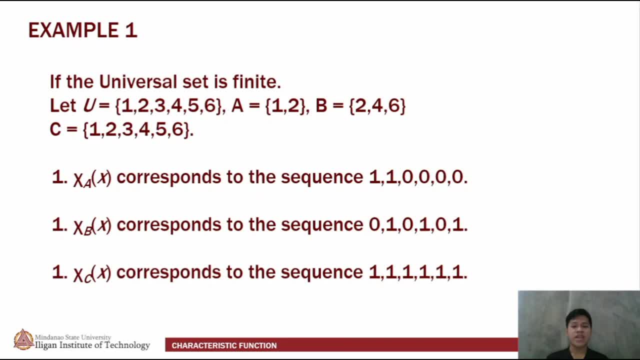 and set A containing the elements 1 and 2,, set B containing the elements 2,, 4, and 6, and set C containing the elements 1,, 2,, 3,, 4,, 5, and 6.. 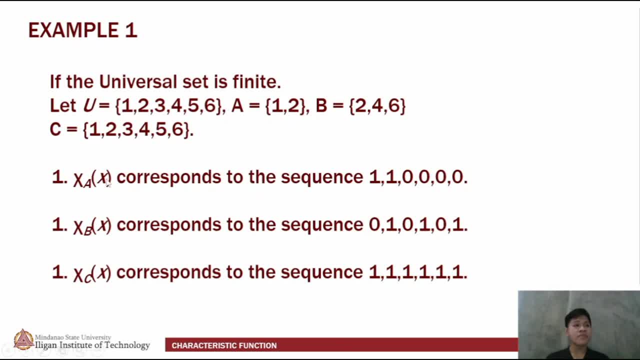 So the characteristic function of the element X on a given set A corresponds to the sequence, Since we are, since we are given that the elements on set A is only 1 and 2, that's why, in this part, right here, 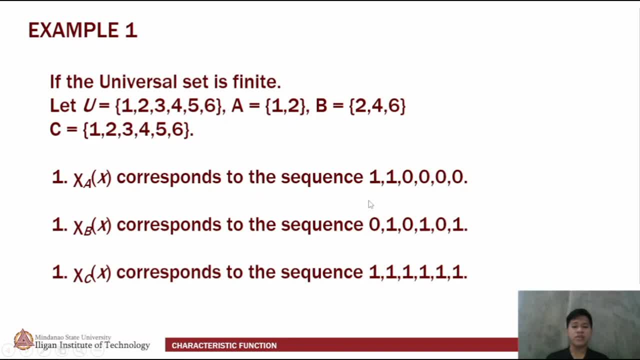 1 and 2 is true, so that is 1, and the rest are 0s. Same goes with B and C, wherein we can see that B only has 2,, 4, and 6, so the sequence goes like 0,, 1,, 0,, 1,, 0,, 1.. 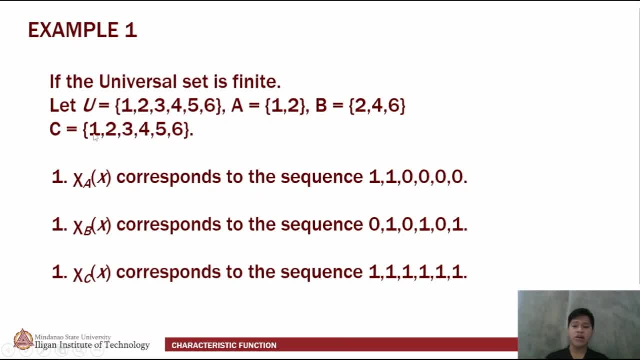 And C. since it all has the element of the universal set, the sequence goes like 1, 1, 1,, 1, 1, 1.. And for the last example, let U be a set containing the elements: 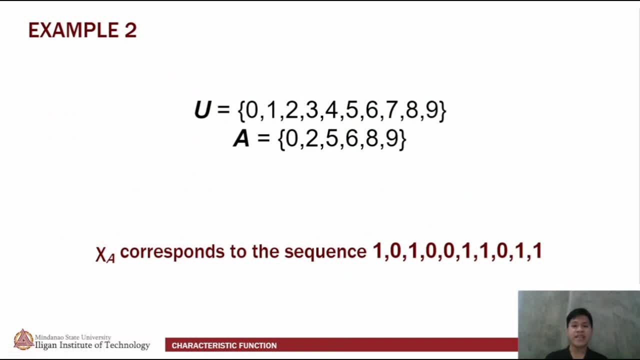 the integers from 0 to 9, and set A containing the elements 0,, 2,, 5,, 6,, 8, and 9.. So the characteristic function for this corresponds to the sequence, Since this is 0,, 1,, 2,, 3,, 4,, 5, and 6,. 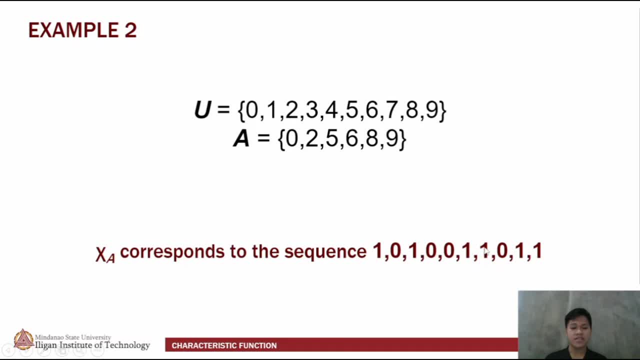 is 0,, 1,, 2,, 3,, 4,, 5,, 6,, 7,, 8, and 9, and the only integers present on set A are 0,, 2,, 5,, 6,, 8, and 9.. 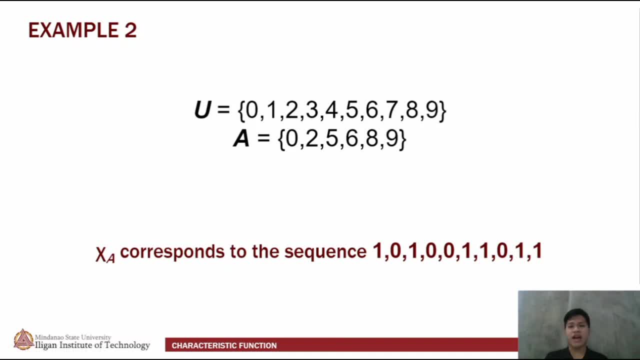 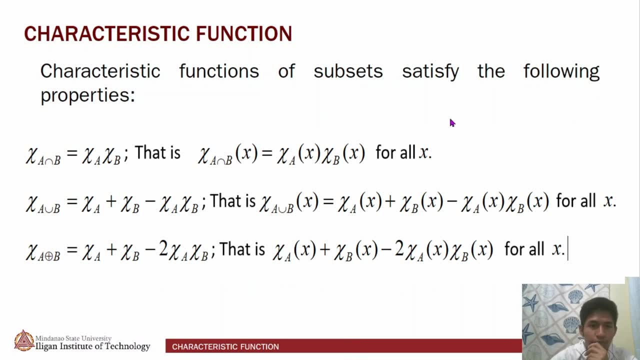 Now for the properties. let's have Anton-Jan report me. So good afternoon everyone. my name is Anton-Jan Legaspi. and for the continuation of the report. so the characteristic functions of subsets satisfy the flowing properties. First, Property 1,. 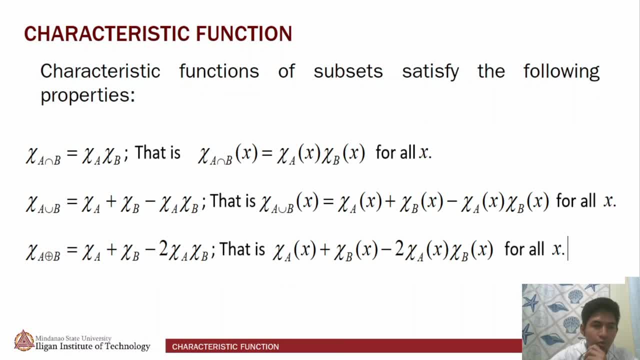 the characteristic function of A- intersection B is equal to the product of the characteristic function of A and characteristic function of B For the property 2,. the characteristic function of A- union B is equal to the sum of the characteristic function of A and characteristic function of B, minus its product. 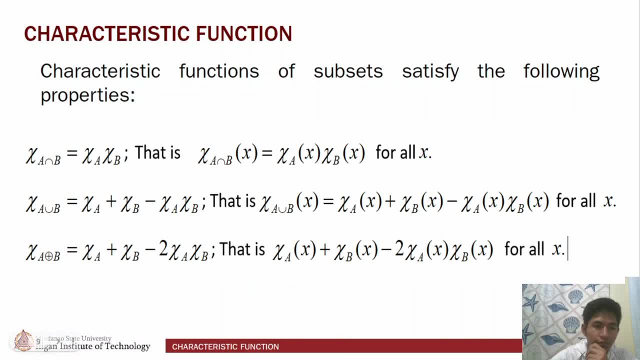 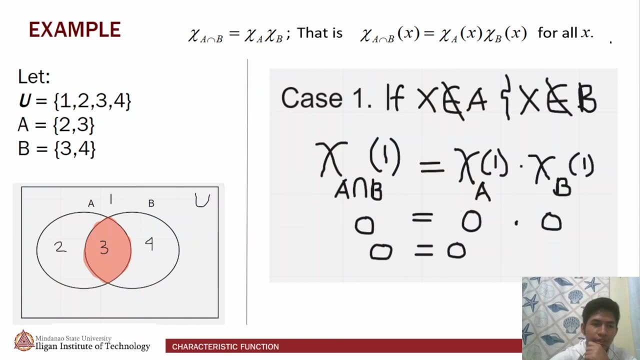 For the third property, the characteristic function of the symmetric difference of A and B is equal to the sum of the characteristic function of A and B, 2 times the characteristic function of a and characteristic function b. so to prove this, let's use an example for case number one for property one, if x is not in a and x is not in b, 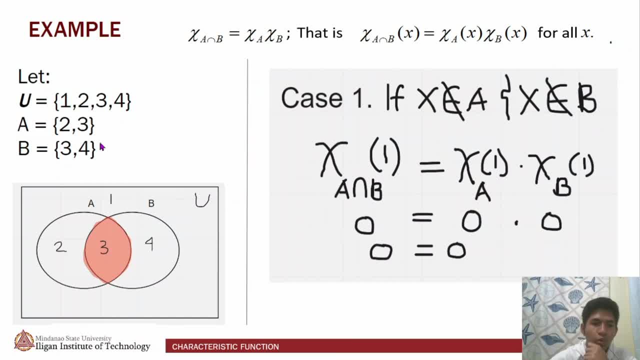 then in this example it referred to the element one. so the characteristic function of a intersection b of one is zero, because one does not belong in the shaded region. then let's prove this referring to this right hand side. so the characteristic function of a of one is zero. 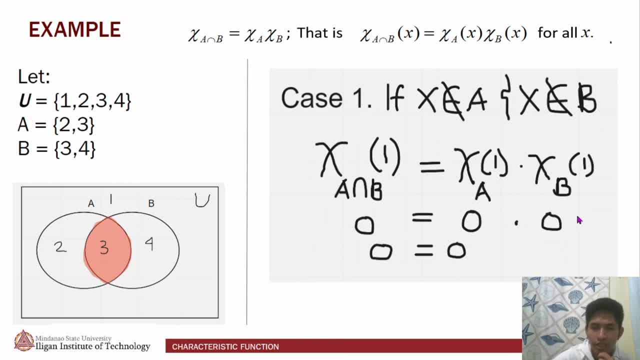 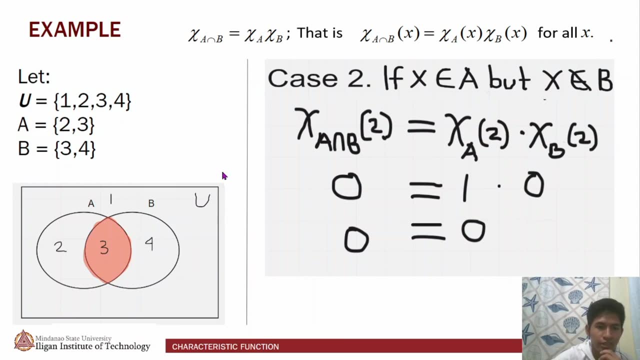 because one does not belong in set a. likewise in set b the characteristic function of b of one is also zero. so therefore its product is zero. and it is true for case number one. for the case number two: if x is in a but x is not element in b, then let's show this. if it is true, so the 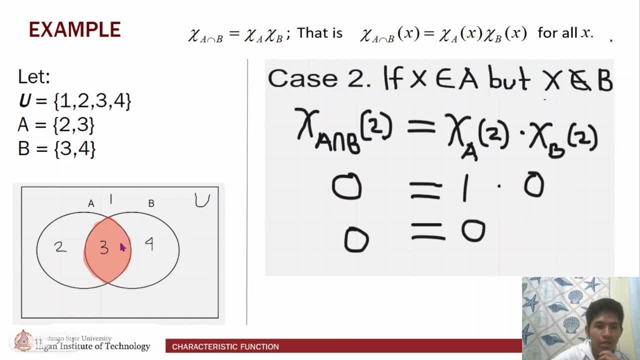 characteristic function of a intersection b of two is zero because element two does not belong on this shaded region, and let's prove this again. if it is true, you're referring to the right hand side. the characteristic function of a of two is one because in set a it contains an. 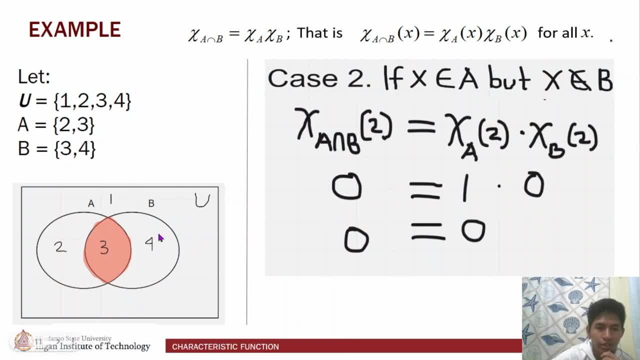 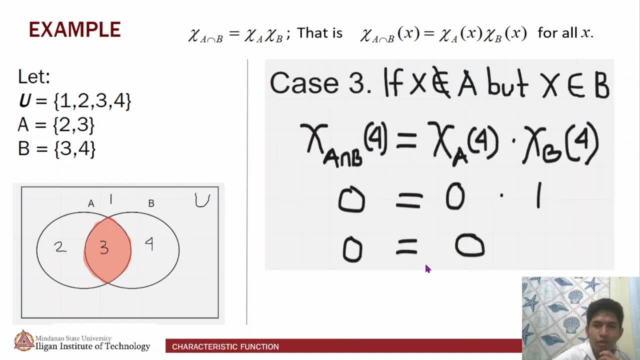 element two. for the characteristic function of b of two is zero, because set b does not contain an element two. therefore its product is zero and it means that it is true for case number two. for case number three, if x is not in a but x is element in b, then the characteristic function 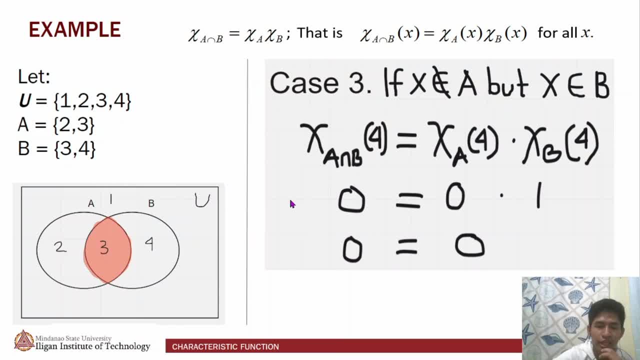 of a, intersection b of four is zero, so in this case it refers to the element four, since four does not belong in this intersection, which means that it is zero. so let's find out if it is equal to the left hand side. so the characteristic function of a of four is zero because in set a 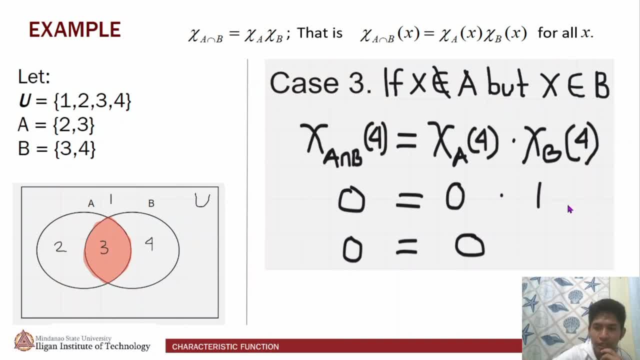 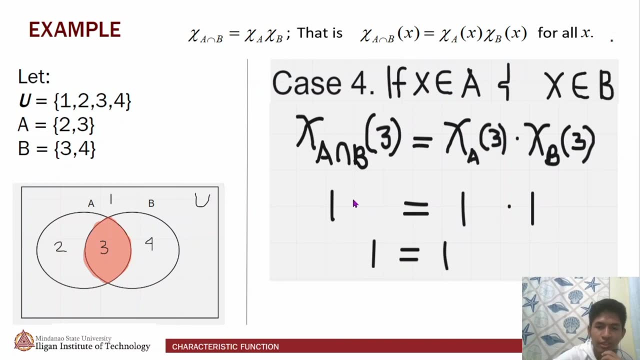 does not contain an element four for the characteristic function of b of four, it is one, because element four belongs to set b, so therefore its product is zero. and it is also true for case number three, for case number four, if x is in a and is also in b, so let's show this, so the 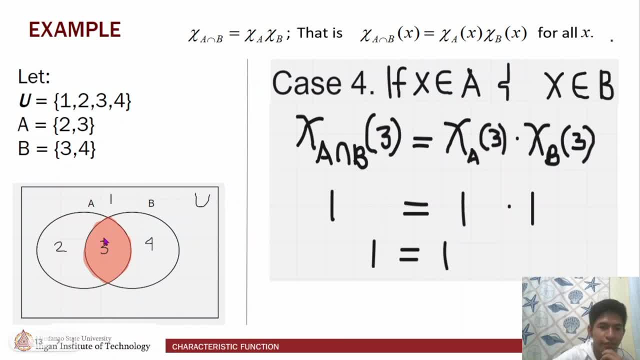 a intersection b of three is one because this case refers to the element three and this element is in the intersection of set a and set b in this shaded region. so let's prove this. if it is equal to the right hand side, so the characteristic function of a of three is one because set a 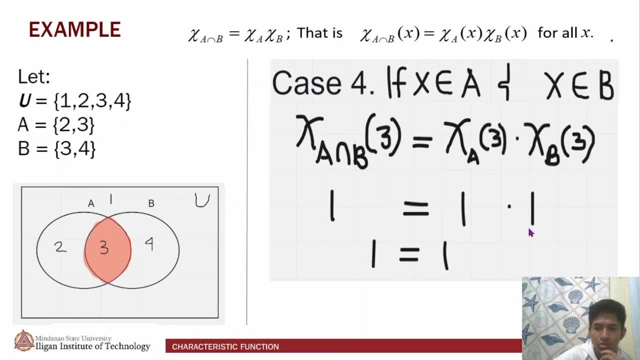 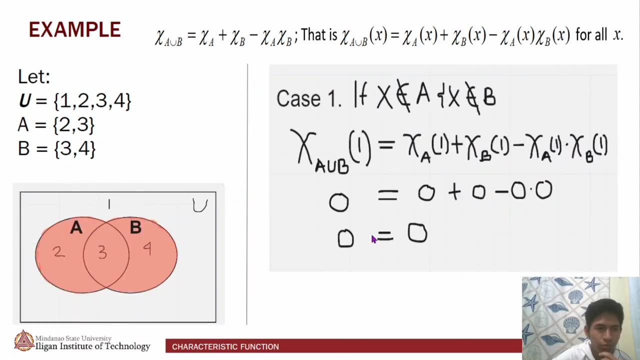 contains an element three and the characteristic function of b of three is also one, because element three is also in set b. so therefore it is true for the case number four and this means that if the cases are true, then it satisfies for the first property. okay, for the property two we have: 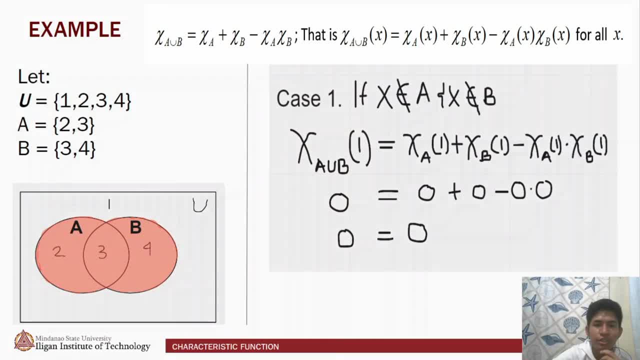 here the characteristic function of a union, b, is equal to the sum of the characteristic function of a and characteristic function of b minus its product. for the case number one, once again, let's prove this using an example. so if x is not in a, then at the same time x is not in b. in this case, 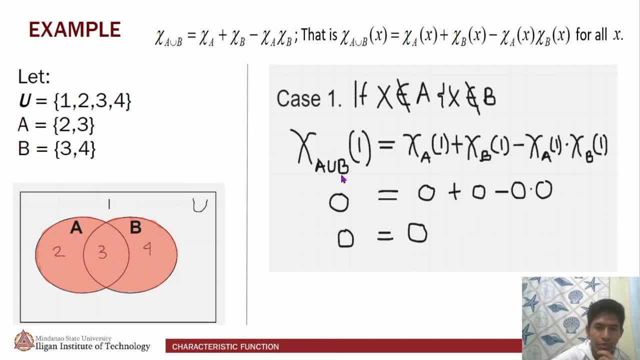 it refers to element one, for the characteristic function of a union b of one is zero, because one does not belong on this shaded region. so let's prove this. if it is true, referring to the right hand side, for the characteristic function of a of one is zero, the characteristic function of b of one is also zero, then its product is zero. 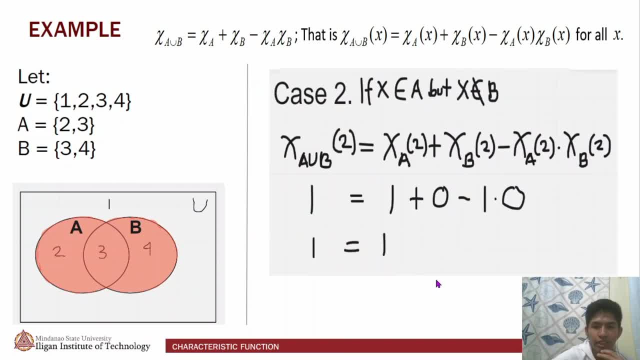 therefore it is zero. it is true for case number one. for the case number two, if x is element in a, but x is not an element of b, so it refers to element two on this example. so we have here the characteristic function of a union. b of two is one, because element two belongs to the shaded. 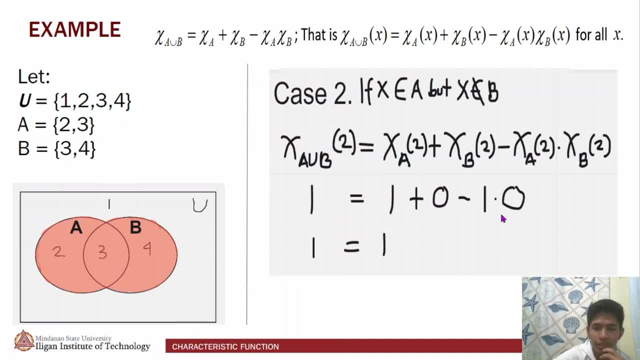 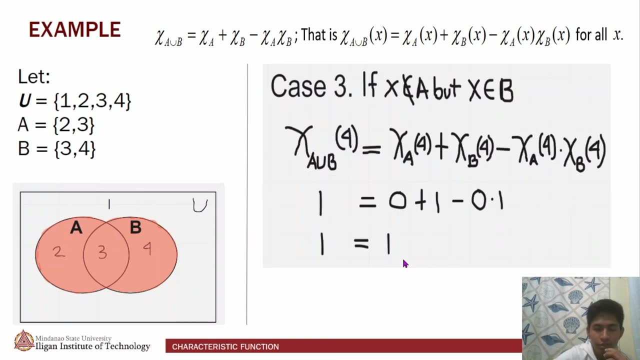 region. so let's show this if it is equal to one using the right hand side. so the characteristic function of a of two is one, because a element two is in city a, and for the characteristic function of b of two is 0 and its product. so therefore 1 minus 0 is 1.. so therefore it is true for the case. 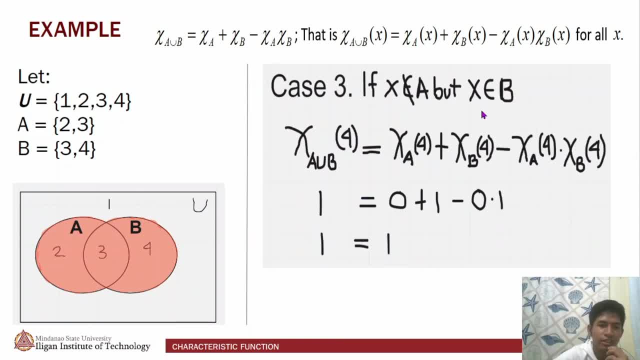 number three, if x is not in a, but x is an element of b. so in this case it referred to the element 4 of a. union b of 4 is 1, once again, because element 4 is inside in this shaded region. so what we have? 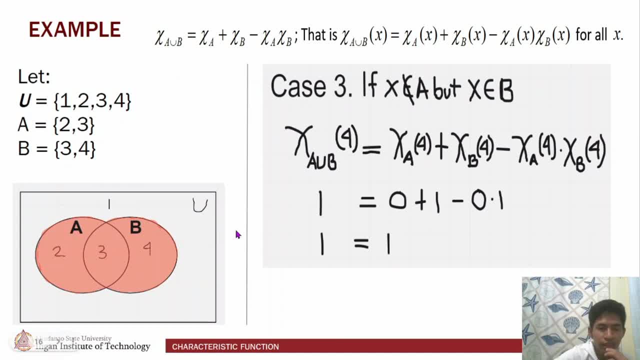 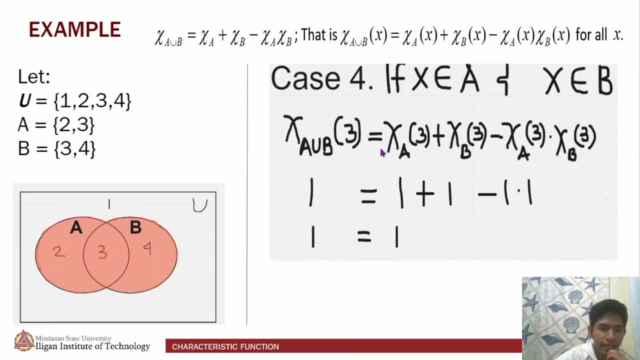 here the characteristic function of a of 4 is 0, because set a does not contain element 4, then the characteristic function of b of 4 is 1, then its product is 0, so 1 minus 0 is 1. so therefore it is true for case number 3. for the case number 4, if x is in a, then at the same time x is in b. 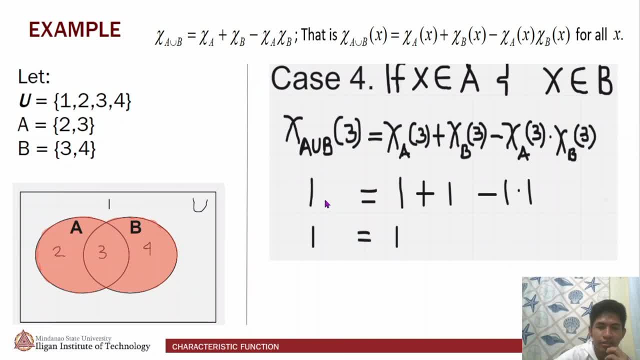 so basically it referred to the element 3. so let's show this: if it is equal to 1, the characteristic function of a of 3 is 1, then the characteristic function of b of 3 is also 1, then its product is 1, then 1 plus 1, 2 minus 1 is 1. so therefore it is true for the case number 4 and therefore, since 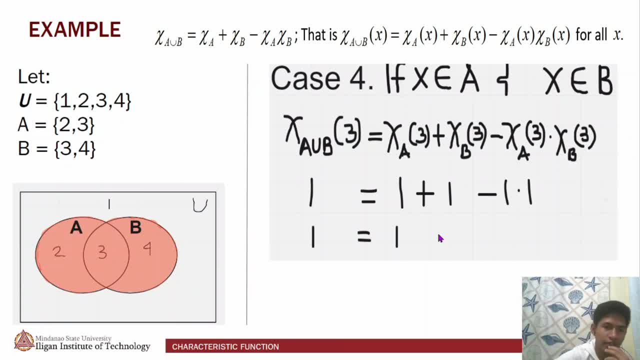 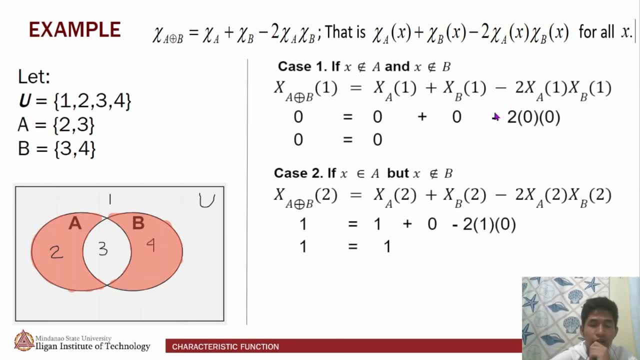 it is true for four cases. then it is satisfied for the second property, for the property 3 we have here, the characteristic function of the symmetric difference of a and b is equal to the characteristic function of a plus characteristic function of b minus 2 times its product. so the idea of the symmetric difference is that you first get the union, then subtract its. 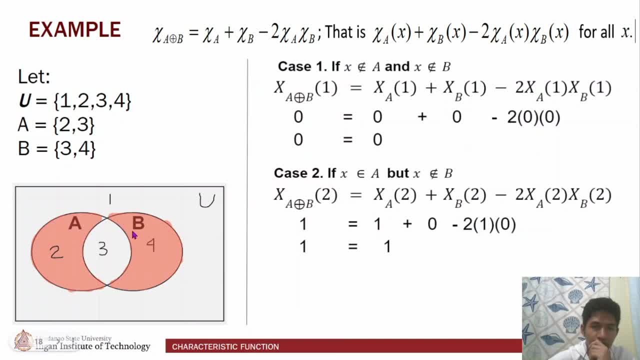 intersection. so basically the shaded region here is the symmetric difference of a and b. so let's back to our topic. so for case number 1, if x is not in a and x is not in b, so it referred to element 1. so for the characteristic function of the symmetric difference of a and b of 1 is 0 because 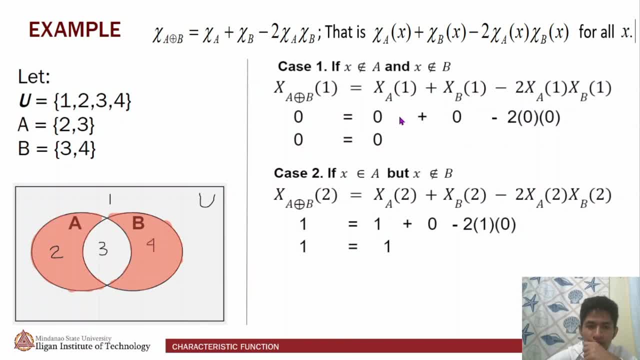 x is not in b, then it refers to the element 2. okay, so what we have here? the characteristic function of the symmetric difference of a and b of 2 is 1. okay, because it belongs to a and b and x is not in b. so the characteristic function of a and b is equal to the right hand side. so the characteristic 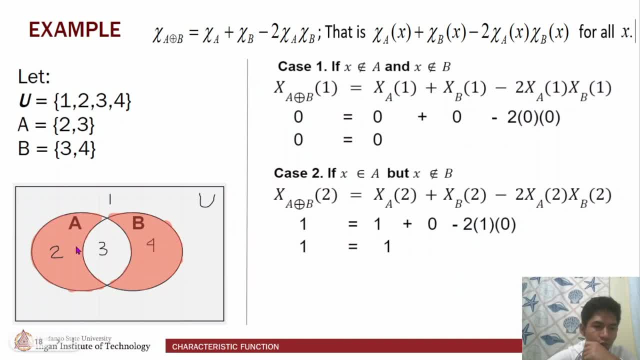 function of a of 1 is 0. the characteristic function of b of 1 is 0 minus 2 times 0 times 0. so it is 0 and it is true for case number 1. for case number 2, if x is in a but x is not in b, then it refers to. 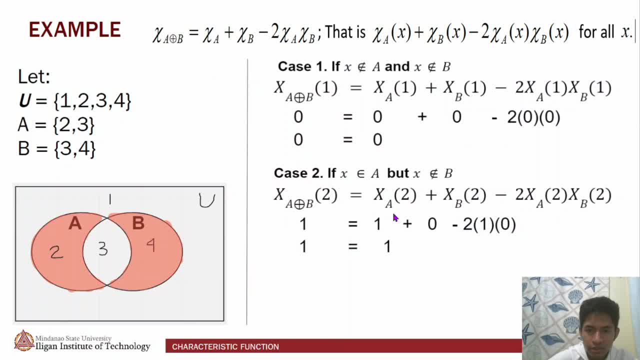 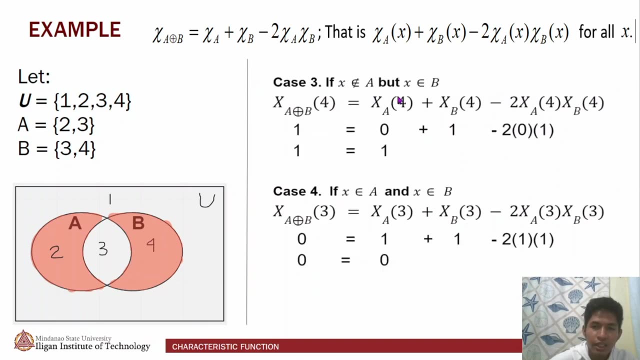 the element 4. so the characteristic function of the symmetric difference of a and b of 4 is 1. so let's show this, if it is true, if it is equal to right hand side, so the characteristic function of a and b of 2 is 1. so the characteristic function of b of 2 is 0 minus 2 times 1 times 0 is 1, so it is. 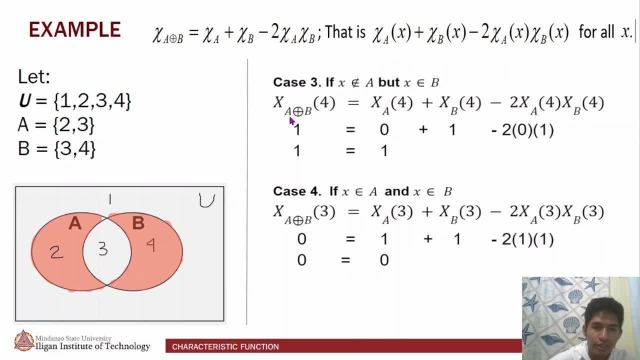 true for case number 2. for case number 3, if x is not in a but x is in b, then it referred to the element 4. so the characteristic function of the symmetric difference of a and b of 4 is 1. so let's. 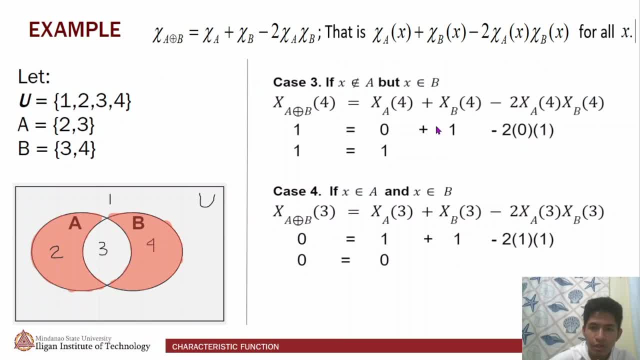 so the characteristic function of a of 4 is 0. the characteristic function of b4 is 1, because it belongs to this shaded region, minus 2 times the characteristic function of a and the characteristic function of b, so it is 0. so 1 minus 0 is 1. so basically, in the case number 3, it is also true.